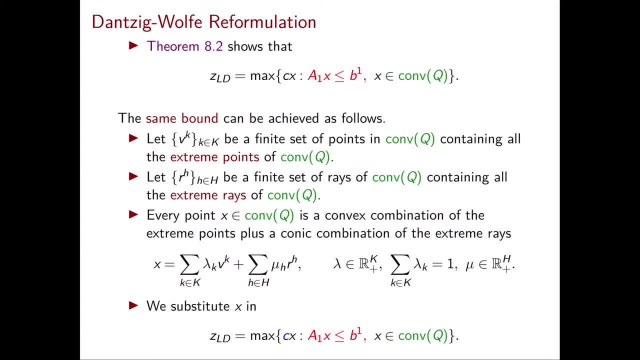 In particular, let vk for k in k be a finite set of points in conv q that contains all the extreme points of conv q, and let rh for age in age be a finite set of rays of the convex hull of q that contains all the extreme rays of the convex hull of q In particular. note that we don't need 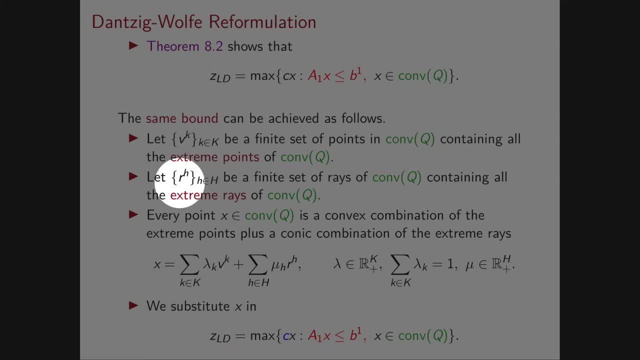 the first set to be exactly the set of extreme points and the second set be exactly the set of extreme rays, but they can be larger sets In any case. then we can write any point in the convex hull of q as the sum of lambda k? vk plus the sum of mu h rh, where 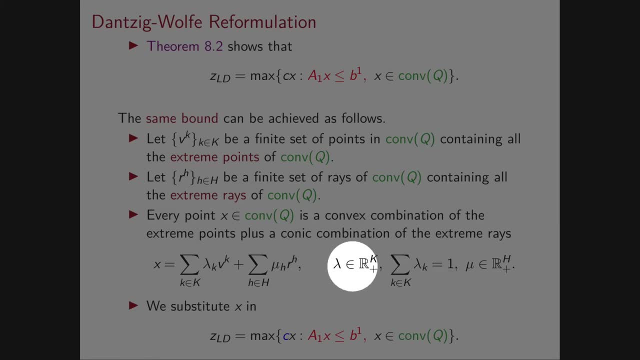 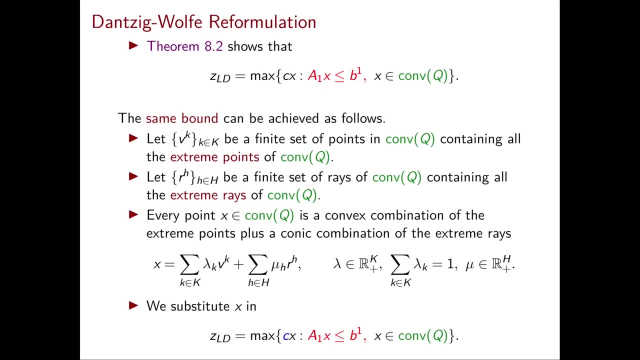 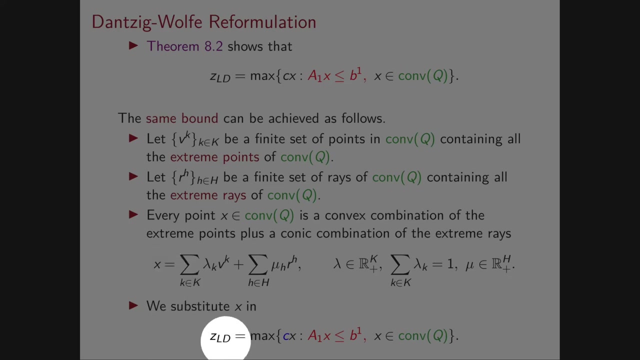 lambdas give convex combinations, so lambda, non-negative. and they sum to one. and mu give conic combinations, so they're just non-negative. In order to obtain the Danzig-Wolff reformulation, we now just substitute the x in the formula for the Lagrangian dual that we saw earlier. so we replace x. 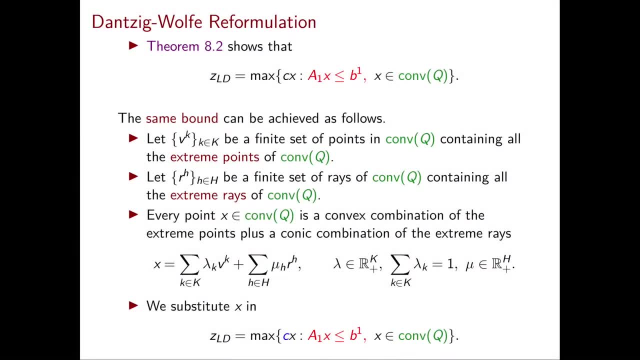 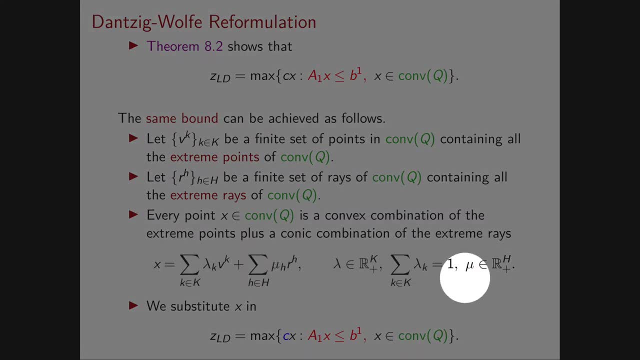 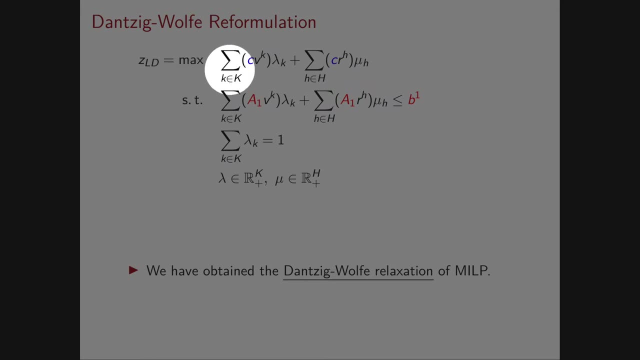 in the objective function and in the constraints, and then we replace the constraint x in the convex hull of q with the constraints that we just introduced. Let's do that. we obtain the following: so zl is the max of. this is the objective function, where we replaced x with the new formula. then 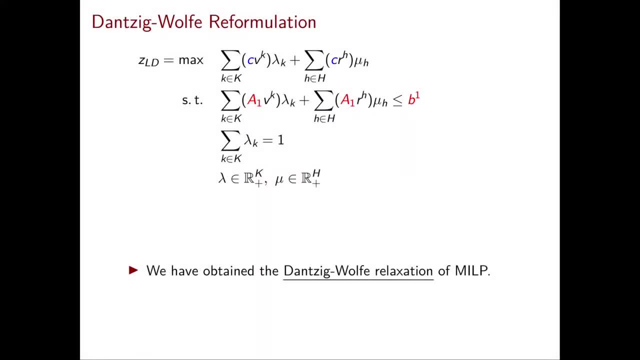 these constraints are those obtained from a1x less than or equal to b1 by again replacing x. and then we have the convex combination and conic combination. This is the definition of the Danzig-Wolff relaxation of the original problem. Note that at this point this is a linear programming. 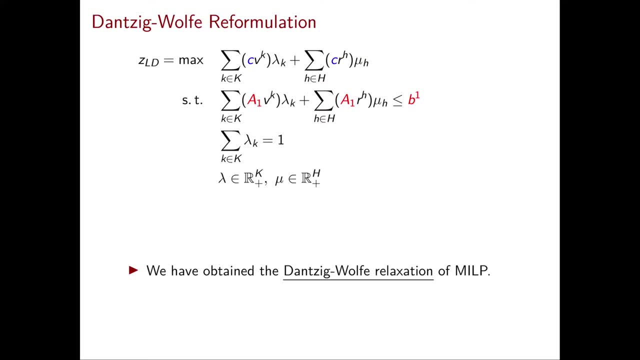 problem and the variables are the lambdas and mu. there's no x anymore. If, instead of a relaxation, we want a reformulation of our original mixed integer linear programming problem, we only need to enforce integrality constraints on the first p variables. We don't have these x variables anymore, so in order to enforce these constraints, we have once. 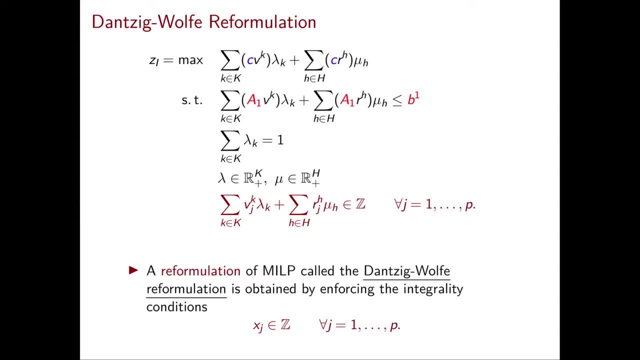 again to substitute x with the formula that we just wrote in the previous slide, and we obtain this condition over here, and this is called the Danzig-Wolff reformulation. What is clear from both the relaxation and the reformulation is that they both have a huge number of variables. 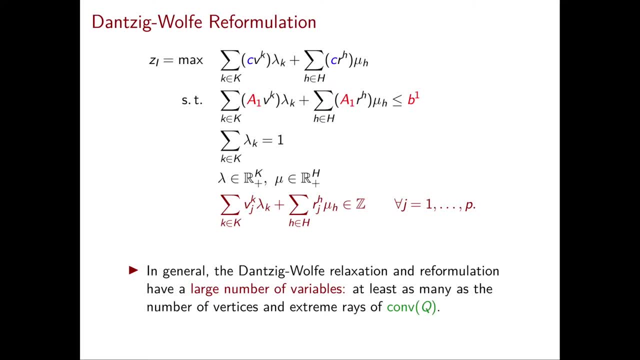 in fact, they have at least one variable for every vertex and for every extreme ray of the convex hull of Q. Let's now consider a setting that often appears in real world problems, and this is the case where the convex hull of Q is bounded. In this case, the formulation at least. 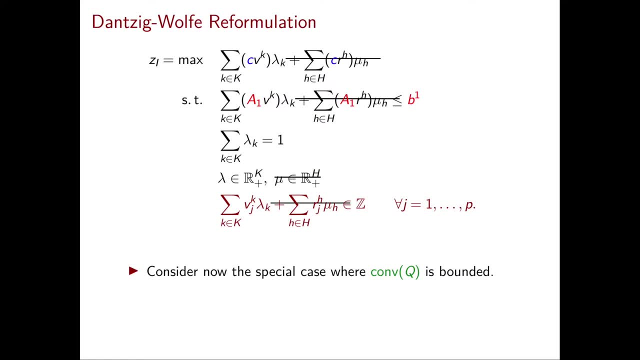 simplifies a little bit, because we don't have any more extreme rays and so we can trash all the part of the formulation regarding the rays R, H and the multipliers mu. If we get rid of all these parts, then the Danzig-Wolff relaxation is not going to be as good as the Danzig-Wolff relaxation. 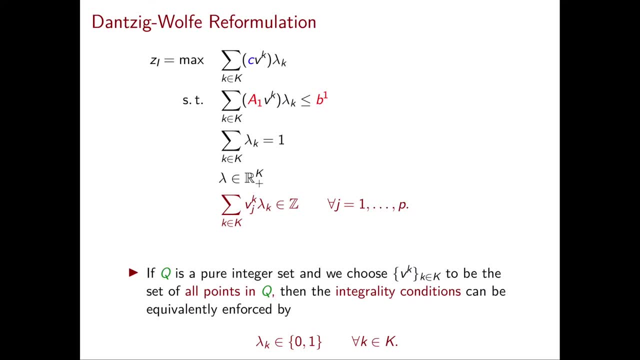 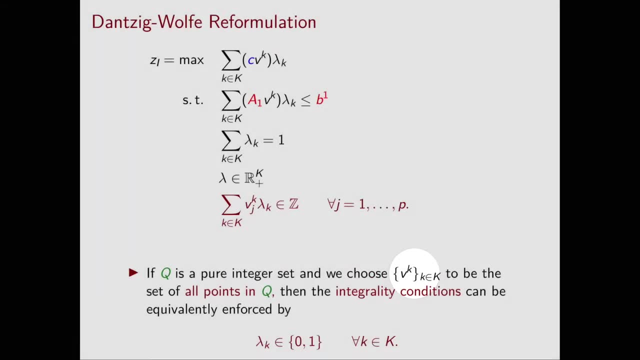 So the Danzig-Wolff reformulation takes this form. And now consider an even more special setting, which is when Q is a pure integer set and we choose the vks to be the set of all points in Q. In this case it's: 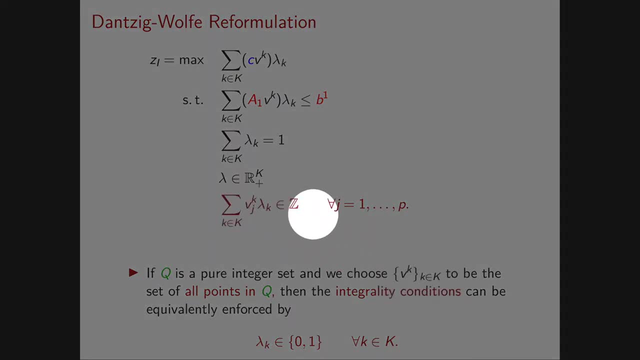 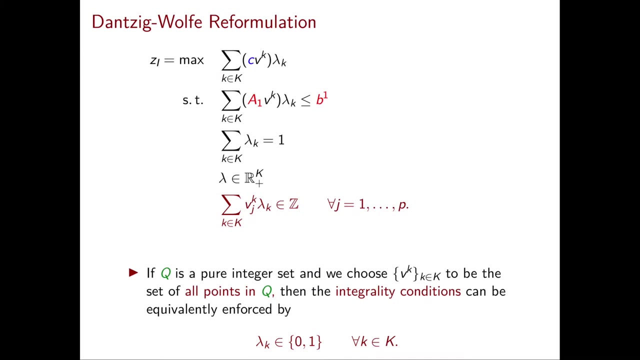 simple to show that the integrality conditions in red over here can be replaced by just the conditions lambda k in for every k in K. To see this equivalence, one should notice that these binary conditions, to get together with the equation sum of lambda k equal to one, will allow only one variable, lambda. 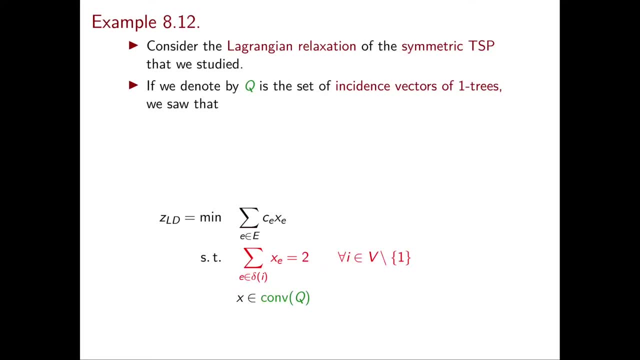 k to be equal one, while all the others will be zero. So let's see now an example, and we consider once again the symmetric TSP and its Lagrangian relaxation that we studied In this example. our set Q was the set of incidence vectors of one trees and our Lagrangian dual took exactly this. 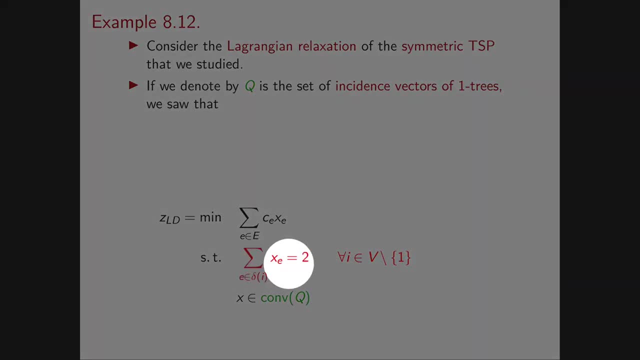 form, In fact our red constraints, degree constraint for every node different from one, And so, by theorem 8.2, the Lagrangian dual is the optimal value of this linear programming problem. So now, in order to write down the Danzig-Wolff: 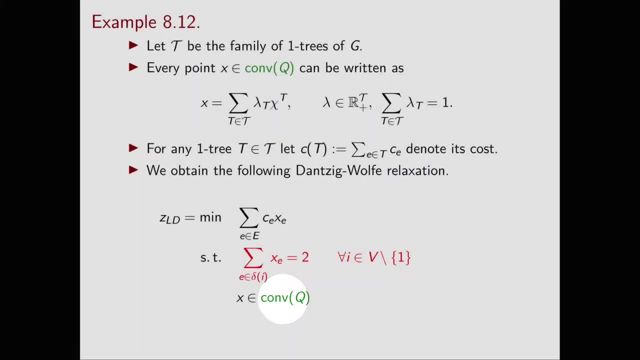 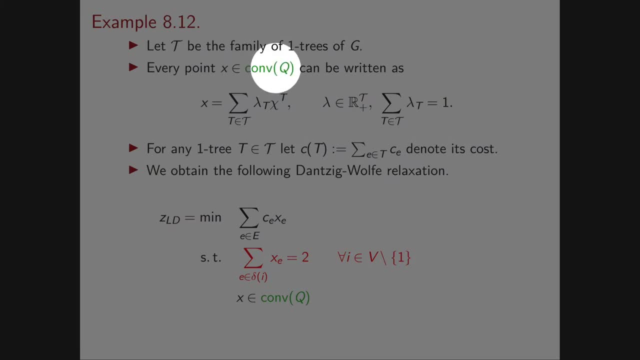 relaxation. we need to write down the vertices of the convex hull of Q, So let T be the family of one trees of G. Then every point in the convex hull of Q can be written as a convex combination of the incidence vectors of the one tree of G, and so let T be the family of one Trees of G. 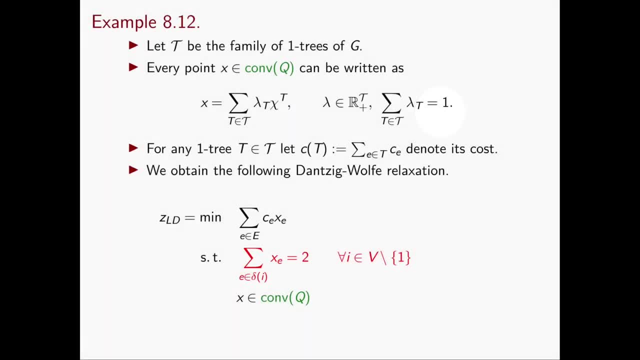 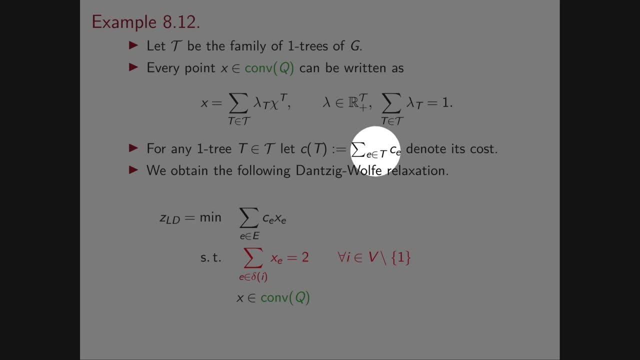 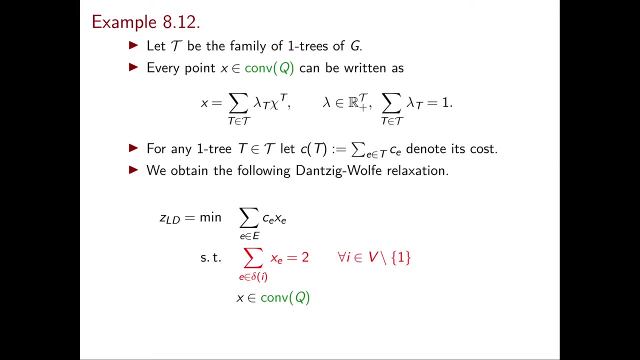 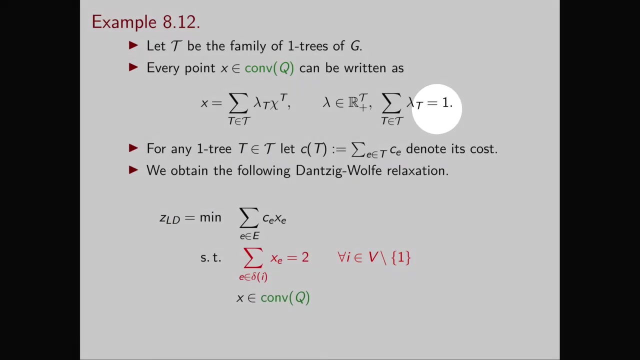 trees of G. therefore X takes this form. now, to simplify the notation, for every one tree T, we use a C of T to denote the cost of the corresponding one tree. then we can replace the X variables in our formulation with the formula that we just obtained and replace X in Q with exactly this condition. so let's do. 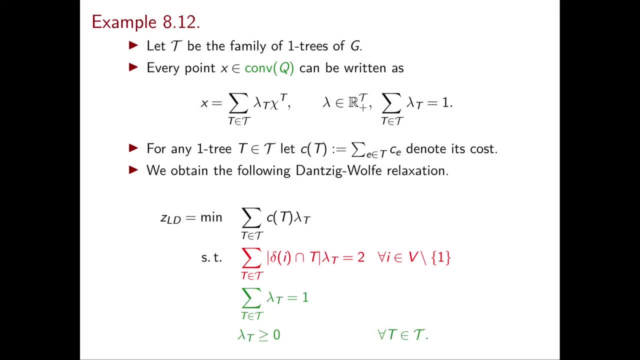 that and that's what we obtain. our red constraints takes this form, in fact, for every T in T, we have that the sum of the XE for E in Delta of I is exactly the cardinality of Delta. I intersected T to obtain the Danzig-Wolfe reformulation. we 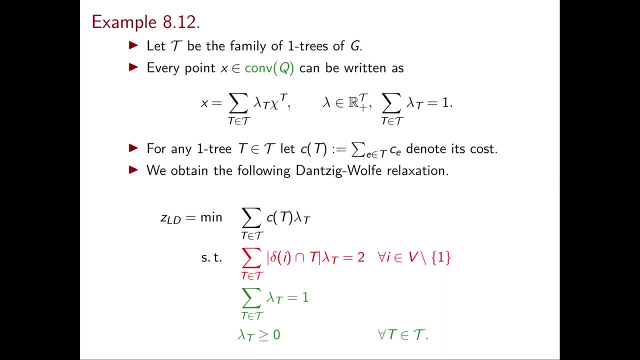 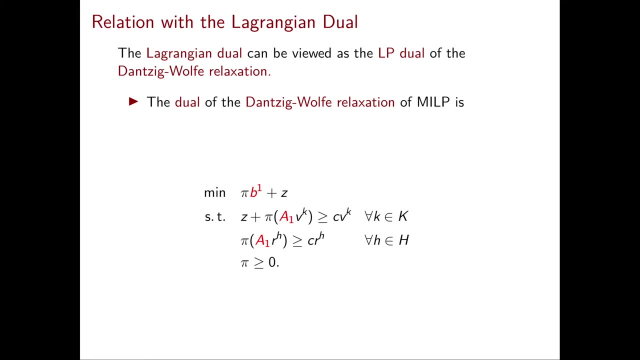 only need to replace lambda T greater than or equal to zero with lambda T binary for every T in T. next, I want to show to you how the Lagrangian dual can be viewed as the linear programming dual of the Danzig-Wolfe relaxation and this argument. 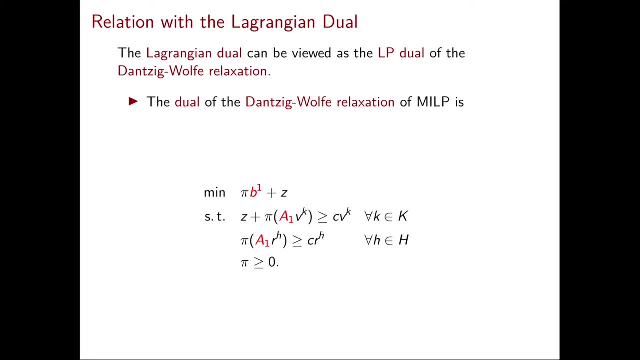 will tie back with our very first observations about the Lagrangian relaxation. so let's look at the Danzig-Wolfe relaxation and let's write down its dual. now you can check that the dual is exactly this minimization problem over here. in particular, the PI variables are associated with the inequalities. 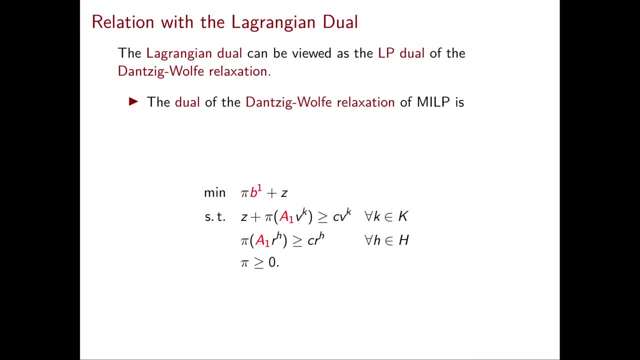 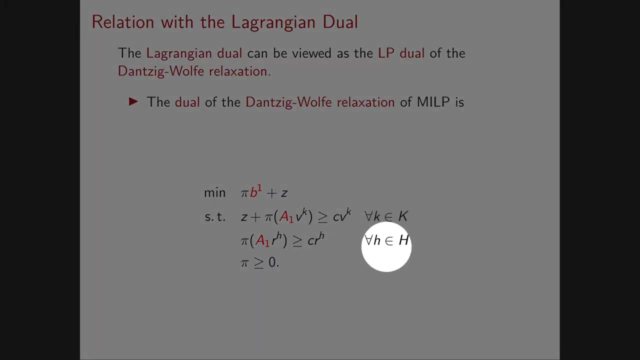 corresponding to the system, A1X less than or equal to B1, and the variable Z corresponds to the equation sum of lambda K for K in K equal to one. our inequalities, of course, correspond to the original variables, so we had one for every K in K and one for every H in H. now the first thing we should notice is: 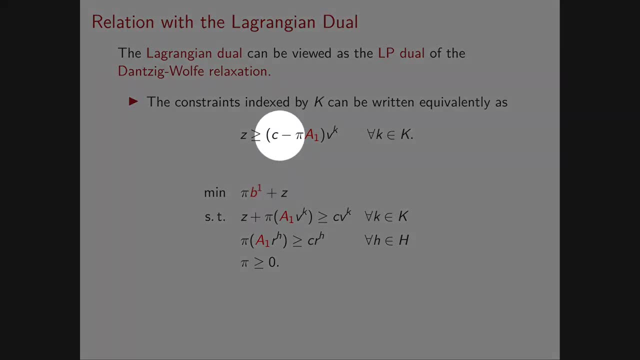 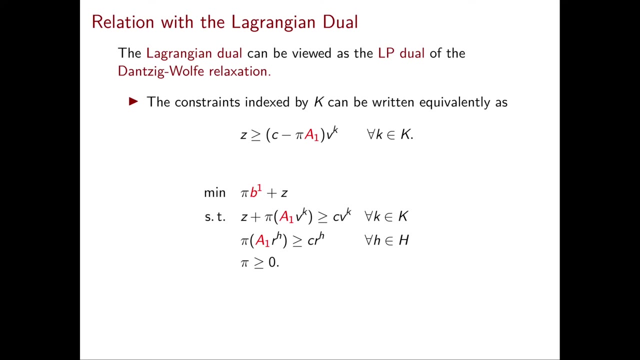 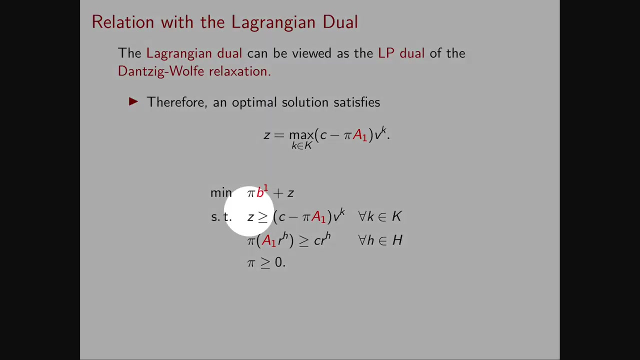 that the first bunch of constraints can be rewritten in the form above. everything we're doing is the leave z on the left hand and bring everything else to the right hand. so let's then replace these inequalities with a new form in this system. here is what we obtain. so now let's examine this. 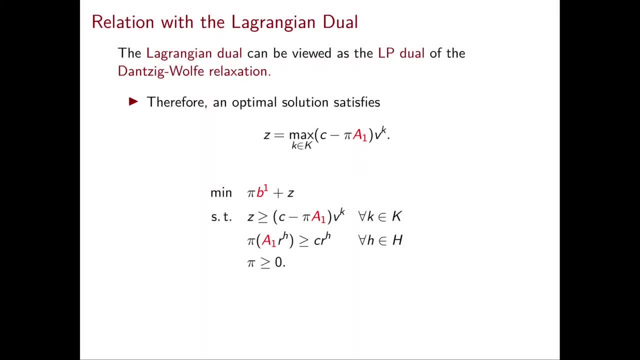 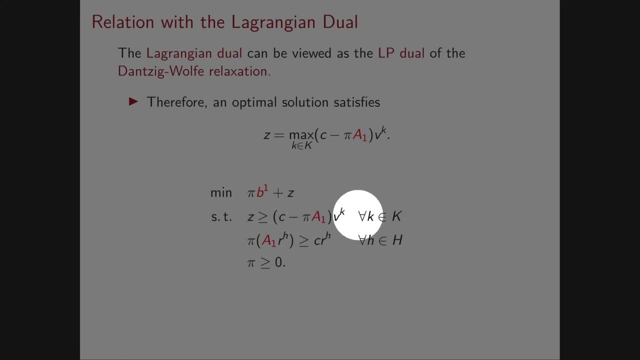 minimization problem and let's see exactly where z appears. so it appears in the objective function. so we are minimizing z and z only appears in this first bunch of constraints. and we have that z must be greater than or equal to a bunch of values. therefore, the optimal z will be exactly the.